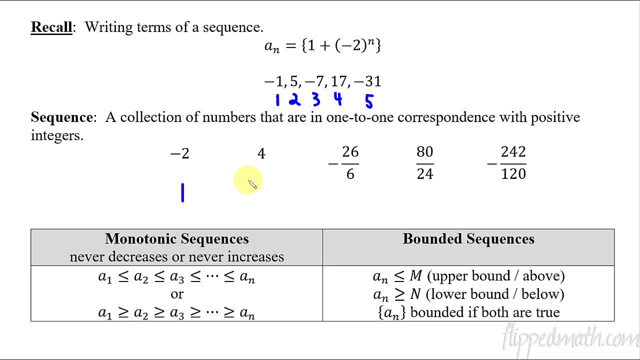 first term, that's a positive integer. the first term is a negative 2.. So this is just a made-up sequence here. I just made up some numbers here. So the second term, the second number in the sequence, is a 4.. The third is a negative: 26 over 6.. So that's the only number. It's not going to be. 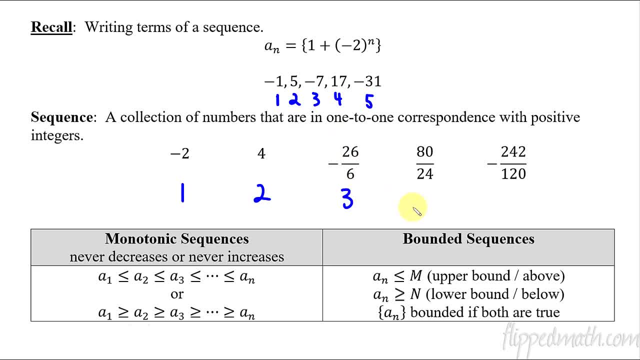 something else. The third term has to be: or the third number in the sequence has to be that number. It can't be something else. That's what this one-to-one correspondence is referring to. All right, so there's the first five terms. All right, so hopefully that is a review of something you've 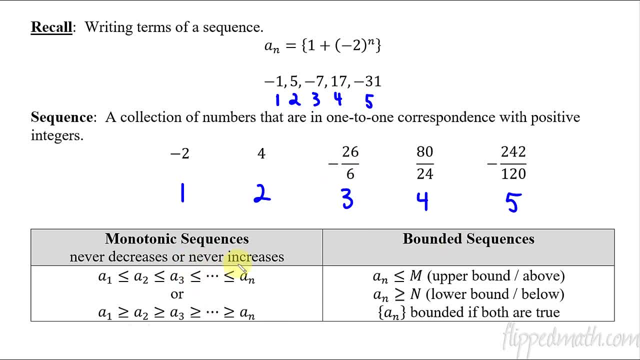 seen before. This is just a sequence of numbers, Now a monotonic sequence. this you might not have heard of before. Monotonic basically means it either never decreases or it never increases. So what I'm talking about is, if I were to graph the numbers, it would be going up, up, up, up. It might flatten out and 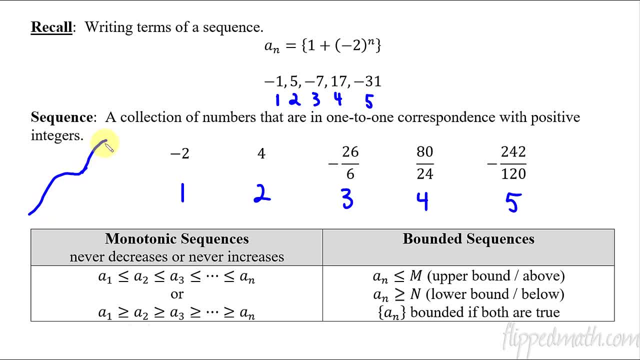 becomes like not increase at all but it's not going to turn around and decrease. That would be considered monotonic sequence, where the numbers just get bigger and bigger and bigger, or start to slow down but still get bigger, or vice versa. It could be getting decreasing, getting smaller and 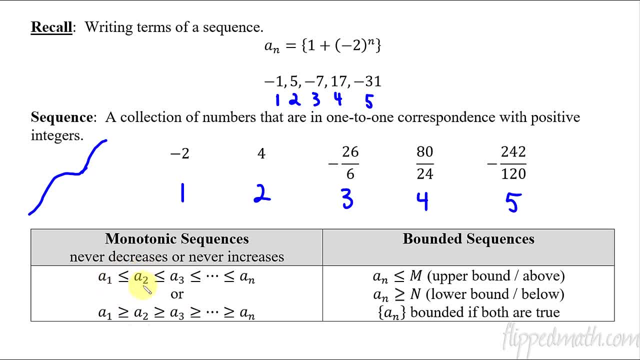 smaller. So you'd say that the first number is smaller than the second number, which is smaller than or equal to the third number, and so forth, until you get to the last term, Or it's larger than the next term, which is then larger than the term after that, which is larger than the next term, and so 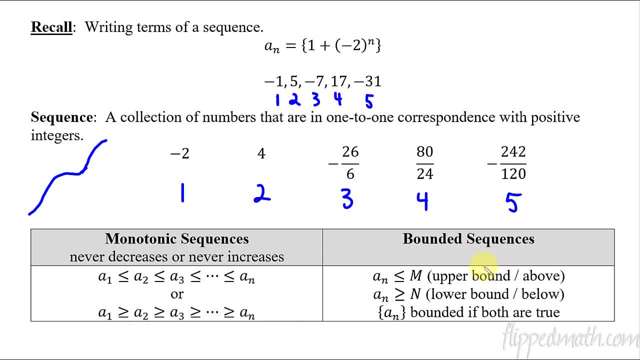 forth. That's monotonic. Bounded is where you have a maximum on the upper bound or a minimum on the lower bound and the whole set of numbers of a, of n, the sequence, the whole thing is bounded if both of these are true. So this is just saying you've got a maximum value. a minimum value is bounded. 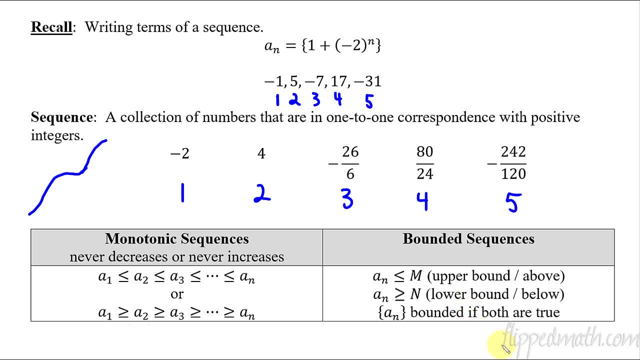 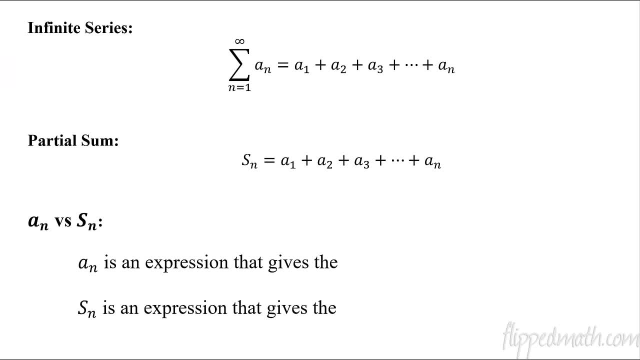 below, and then if it's bounded on top and bottom, then the whole thing is considered bounded. Okay, so now this leads us to our next group of things, Which is infinite series and partial sums. So an infinite series is when you have a sequence of 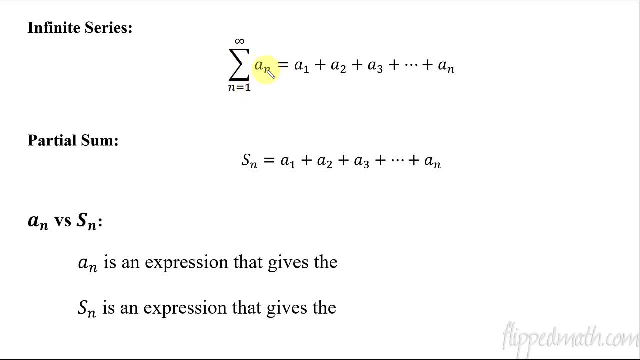 numbers and you're adding them all up. So you have the first term, the second term, the third term, the fourth term, the fifth term, and how many terms? All the way up to an infinite number of terms, and you're adding them all up. That is an infinite series. Now, some of you'd be thinking 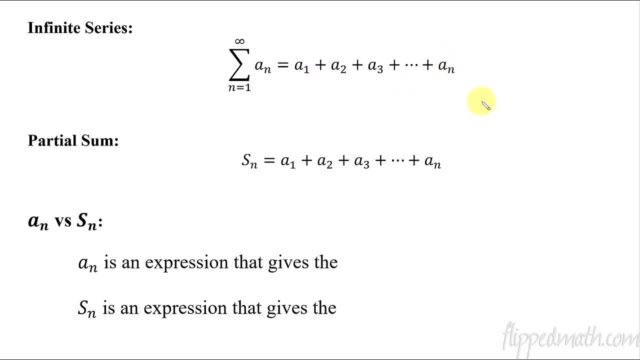 if you're just adding all these numbers up, isn't that just gonna go to infinity? Not always. Sometimes, yes, but not always. So you're gonna see what we're gonna say. If it went off to infinity, that would be considered diverging, which we'll discuss Now. a partial sum: 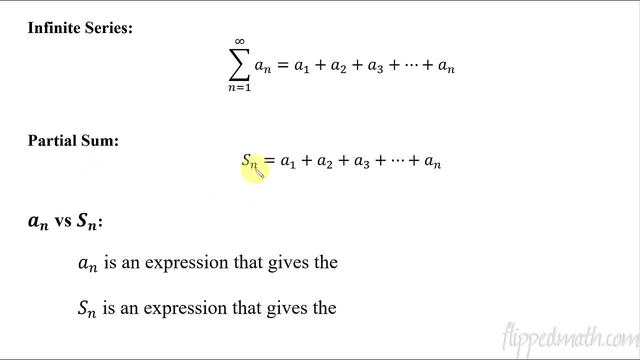 is where you take the sum of the first n terms. So like if I said the first five terms s of five, that partial sum would be the first plus the second, plus the third, plus the fourth plus the fifth. That's what s of five would be, adding up the first five terms. So that's a partial sum. So 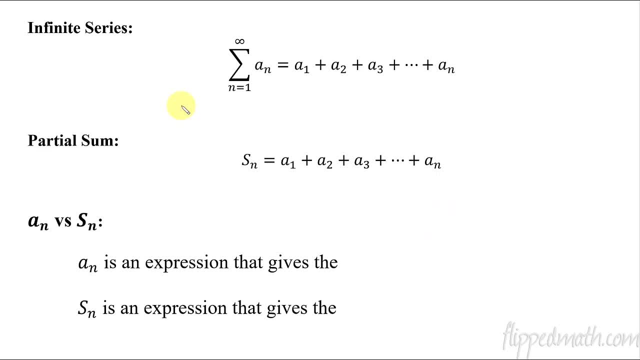 the difference between them and this is important for you to understand to be able to answer questions correctly. a of n is an expression that gives the nth term in a sequence. s of n is an expression that gives the sum of the first n terms of the sequence. So you see the difference. a of n is a specific term. 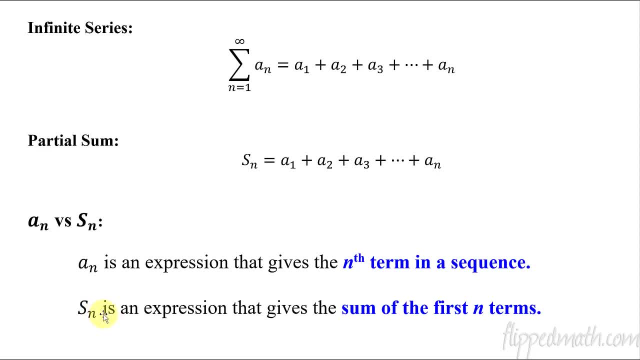 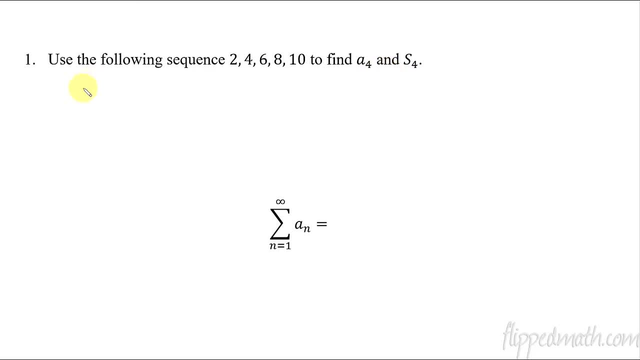 s of n is the addition of all of the terms up into that number. So get that written down and let's do a quick example. So let's find a of four and s of four. a of four, really simple. a of four is just. 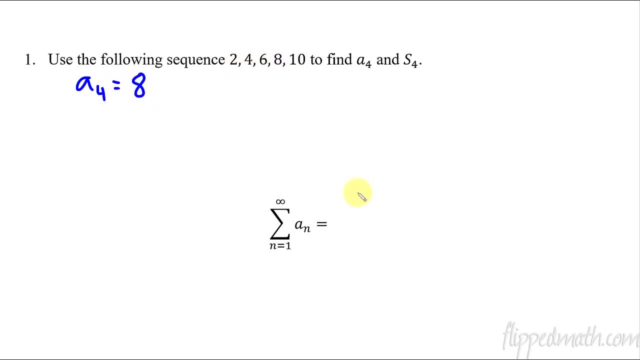 the fourth term: one, two, three, four. It equals 8.. Whereas s of 4 is equal to the first four terms added together. So it's two plus four plus six plus eight. Add those all together ten twenty, you get 20.. 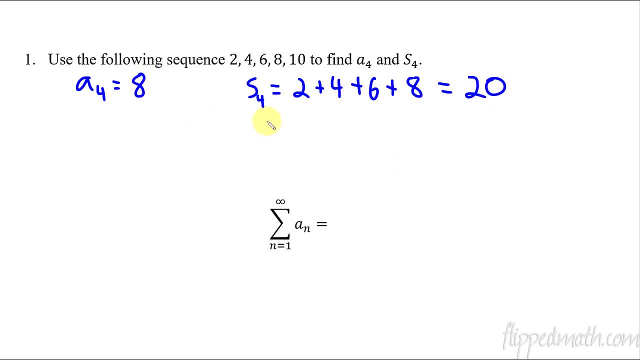 So you see the difference. a of four is only the fourth term, s of four is the addition of all of the first four terms. adding up. Now that leads us to: if you have an infinite series, so you you do the summation. 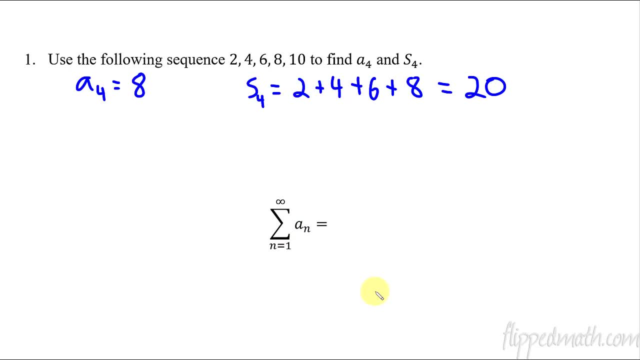 of of the terms a, of n up into infinity. that is exactly the same thing as saying: you take s of n and you have n approach infinity, the limit as n approaches infinity. so now we're going back to limits again. these two things are equivalent and that's an important thing to understand, because sometimes 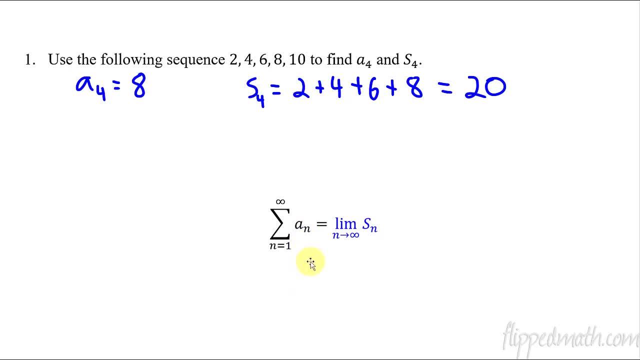 you, the problem might give you a of n or the problem might give you s of n, and you have to understand which they're talking about and that if you have to find this but they only give you s of n, then you just got to know. oh, i'm just taking n, as n approaches infinity of s of n. okay, you'll see. 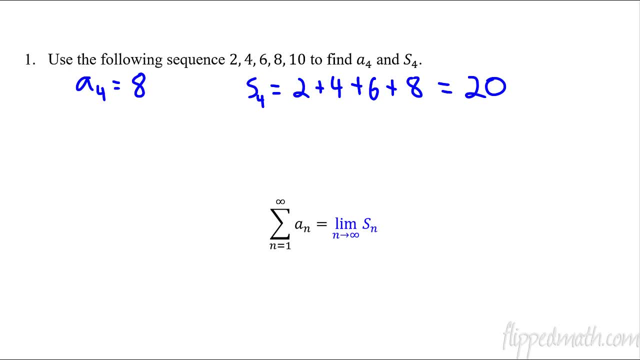 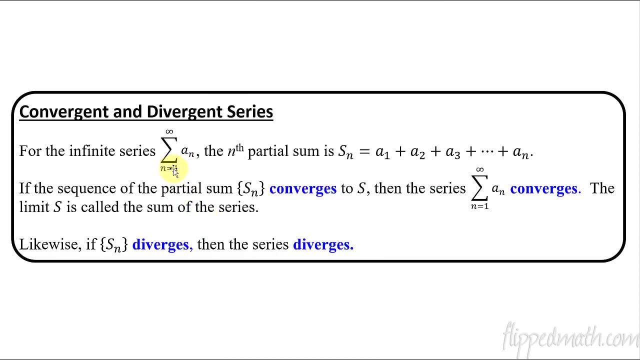 here with a couple examples. we're going to do all right. now it's definition time. so we have convergent and divergent series. so for the infinite series of n to infinity of a, of n, the nth partial sum is this. we've already talked about this, that's the partial sum. 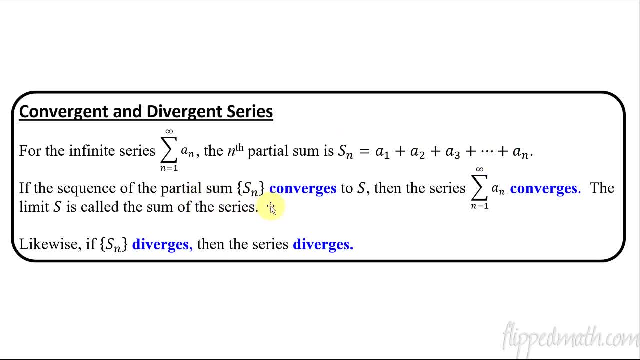 if the sequence of the partial sum meaning, and when i say the sequence of the partial sums meaning you look at s of 1, then you look at s of 2, then you look at s of 3, then you look at s of 4, s of 5 and so forth, so 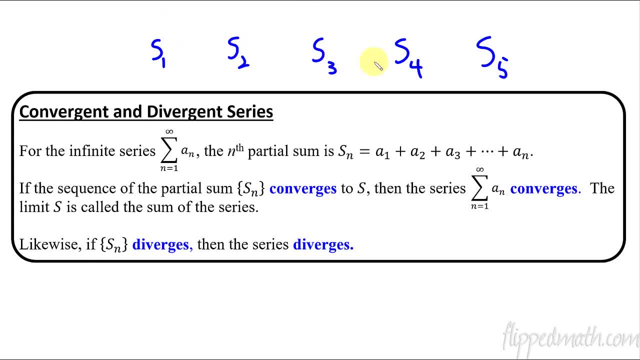 you're adding up the first term, then you look at the next term, then you look at all of these, so you just keep looking those. if those numbers are getting closer and closer to a specific number, if it converges to s, if it approaches a specific number- that's what this is- then the series also. 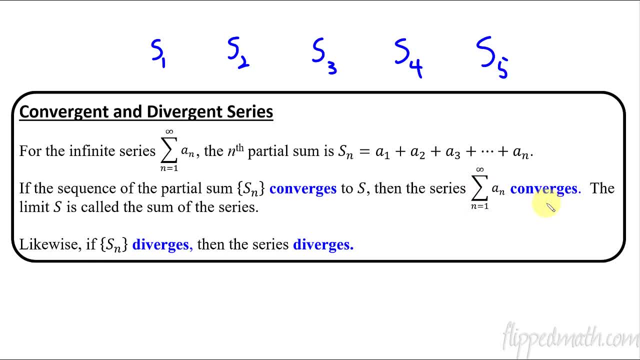 converges or approaches a certain number. that same number s i, and that s is kind of confusing, like maybe i should have used a different letter letter there. it's just saying we're going to approach a specific number, converge to a value. so then the limit s is called the sum of the series. 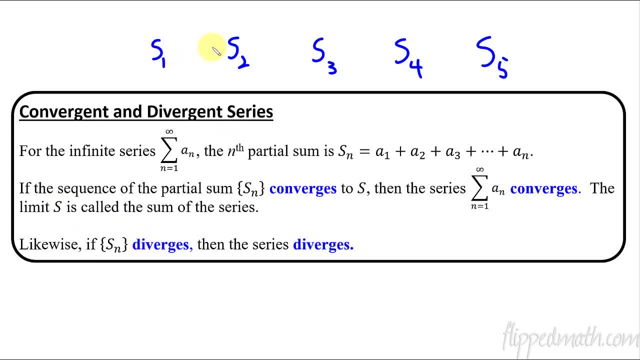 now the likewise. you can do it the other way if, if it diverges. so if you look at these partial sums and you're adding them all up and they don't seem to be approaching a number at all as you get larger and larger and larger, then it's diverging, okay. so and if s of n, if s of n is diverging? 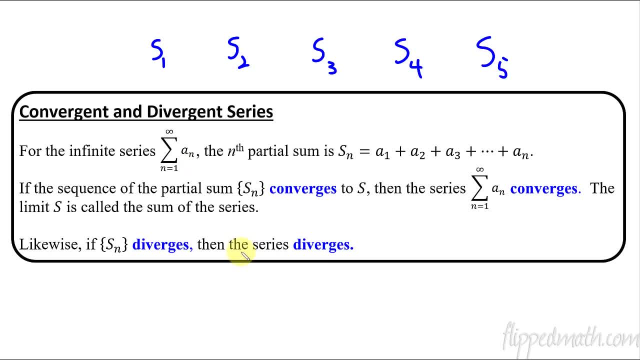 then the series is also diverging. all right. so basically, when we try to answer this, we really look at the partial sums. That's what we're trying to figure out, what the infinite series is doing. Okay, So let's look at the first one. Does the series 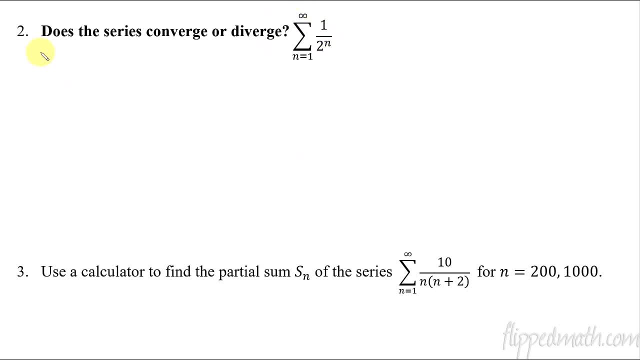 converge or diverge for this. So the quickest way to start doing this is: let's look at: S of one First term is going to be: the sum of the first term is just one over two. You plug in a one because, remember, this is your A of N. All right, Well, that doesn't tell us much. Let's look at: 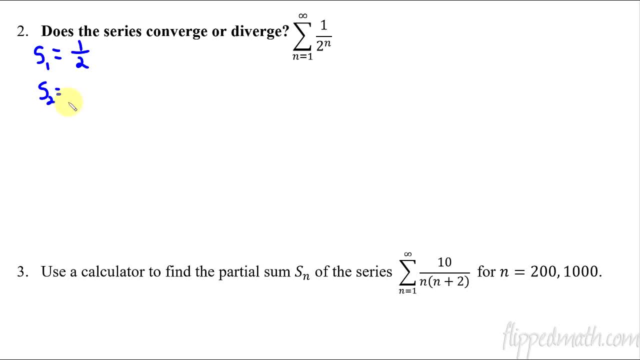 the next one. The second term is going to be the sum of the first two terms, So it's the first term, which is one half, plus the second term, which is plug in a two, You get one fourth, All right. Well, one half plus one fourth is three fourths, because I'm doing this in my head. All right Now. 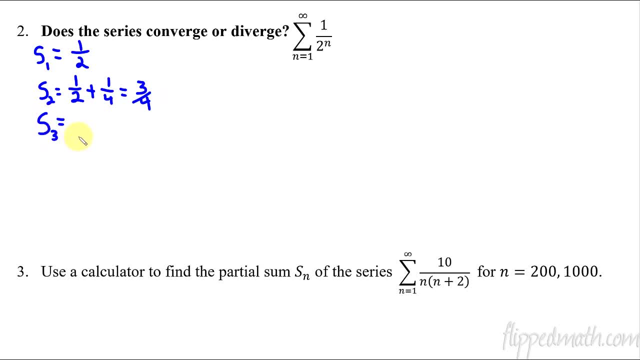 that's good. Let's look at the third one. The sum of the first three terms is going to be the sum of the first two, which is three fourths plus the third term, And the third term is one over two to the third one eighth, And then that equals three, six, seven, seven, eighths Trust. 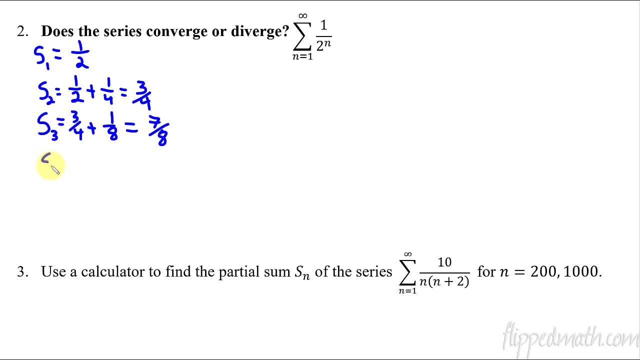 me on that. I know my fractions. And then let's do this fourth term. We'll stop after the fourth term. So the fourth term is going to be the first three terms added together, which is seven, eighths, plus the fourth term, which is one over. two to the 16th, two to the fourth. excuse me, That's. 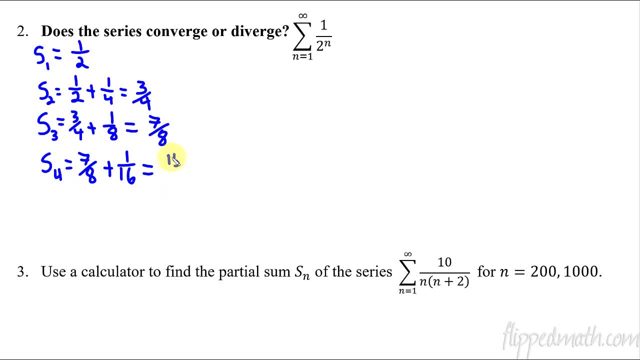 just 16.. And then add it all up, That equals 15, sixteenths. All right, So look at the sequence of two to the fourth. So the first term is going to be the first three terms added together: the sum, these partial sums. the partial sum is one half, The next one is three, fourths. The next 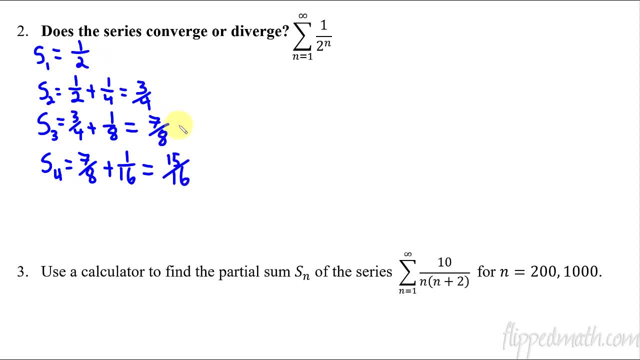 one is seven eighths, The next one is 15, sixteenths. Can you see what number it's getting closer and closer to? It looks like it's getting really close to the number one, So I would say it's probably converging. but that would just be a guess on my part. It looks like it's converging. 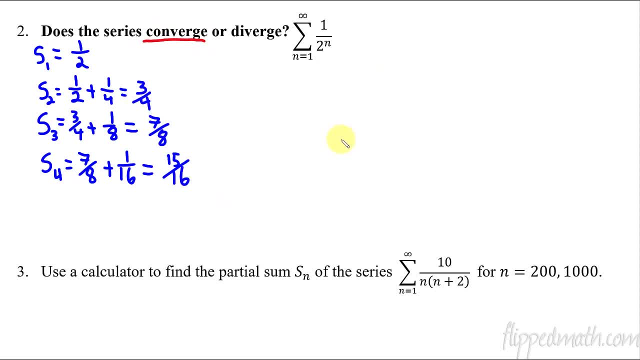 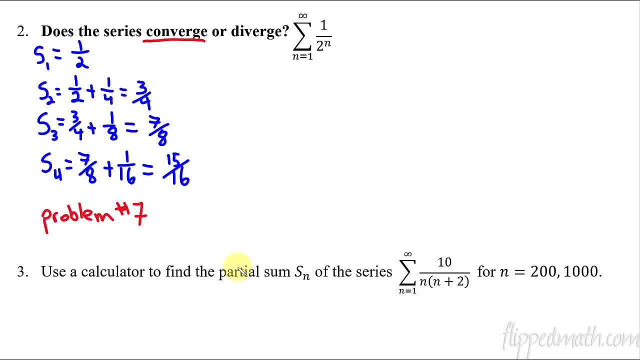 problem number seven, And there will be a problem like this on the mastery check. So please pay attention to what I'm about to do. I'm going to show you how to figure out what S of N is, because if we know S of N is a ton easier. Why? Because if we know S of N, we can just take the. 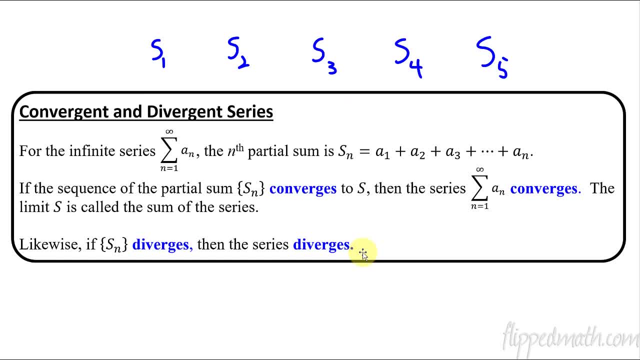 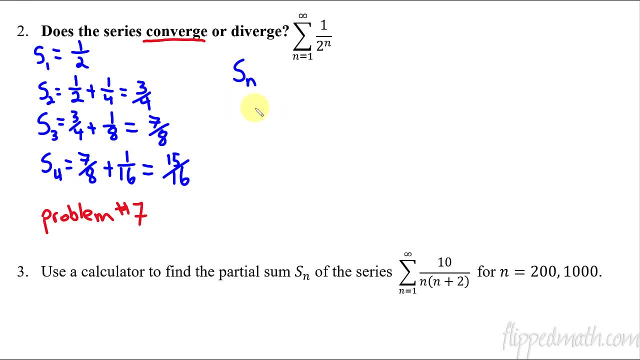 limit as N approaches infinity, and then we're done. So knowing S of N makes this a lot easier. if you can't see it from the partial sums, Okay, So it just depends on the strategy of the problem for these ones that we're starting off with. So this is going to be, so here's the. 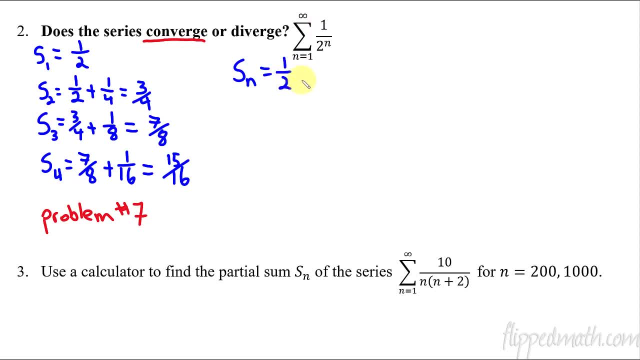 strategy. how you do this. You write out the first term, one over two to the N, plus I'm going to write out the second one. but I'm not going to simplify it, I'm just going to plug in the two right there, Plus I'm going to write the second one but plug in the three. That's the excuse. 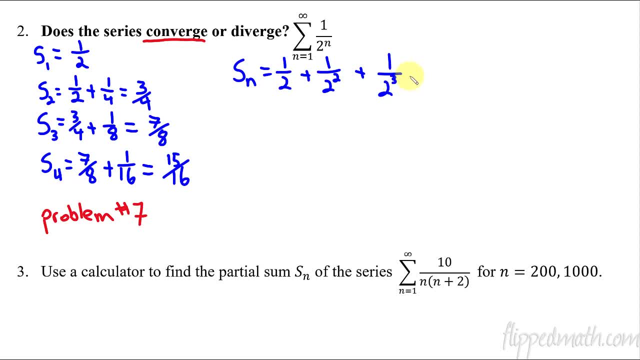 me, I mean the third one. So the third term is one over two to the third plus, And then you could just keep going until dot, dot, dot, until you get to the last term, which is one over two to the nth power. All right, That is S of N. So how can we make a rule out of this? You focus? 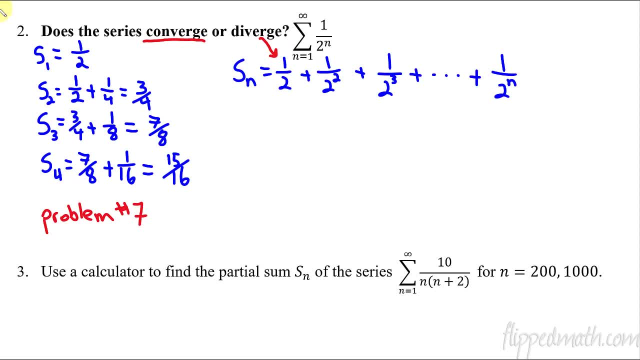 in here on this first term. that term is a one half. What I'm going to do is multiply both sides by one half. So if I multiply the left by one half, I get one half S of N, and then that equals. 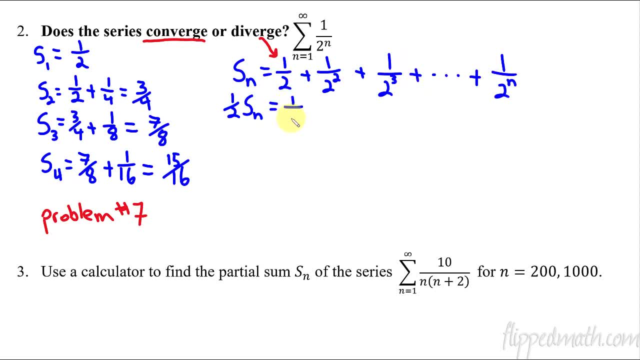 and now I'm multiplying every single one of these terms by a one half, So that makes this become one half squared, plus one over two, cubed, plus one over two to the fourth, plus dot, dot, dot all the way up until we get to the last term. 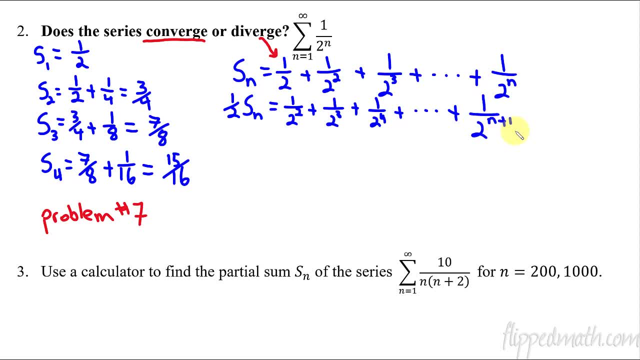 then be two raised to the n plus one. It's one more because I have an extra one half in there. All right, Now that you've done this, you subtract these two lines. So again, you're going to do this again on problem number seven. So you refer to this example. So we say S of N minus one half S. 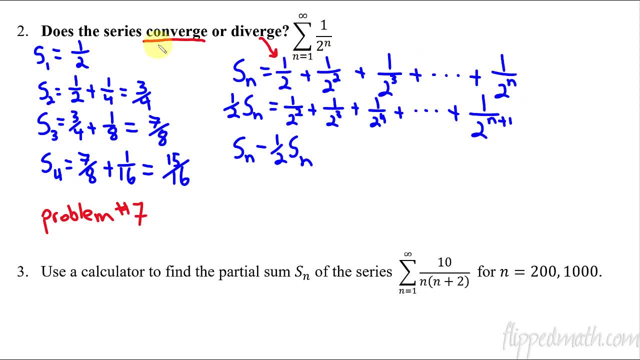 of N. We're going to take this full line and subtract this full line. Well, if you do that, notice what happens. You have this is going to be subtracting from this one and they cancel. This one over two to the third is going to cancel with this one over two to the third. 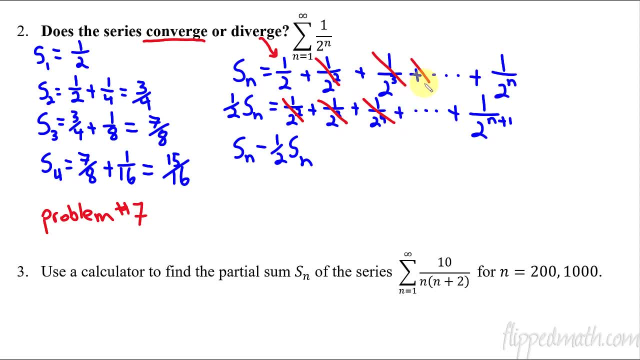 because you're subtracting this bottom line And so that one is going to cancel with the one over two to the fourth all the way up, And then this one's going to cancel with the one over two to the N. that was there. They're all going to start canceling And the only things you have left that 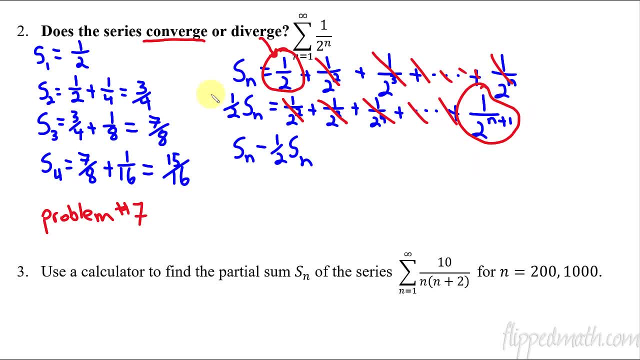 didn't cancel was for these two terms. So we're going to write out that this equals one half, and then we subtracted this line right, So it's minus one over two to the N plus one. So in a simplify, the left side, that's just one half s of n equals one half minus one over two to the n plus. 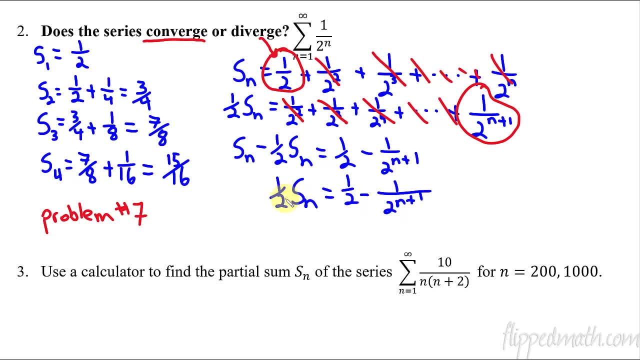 one. now multiply both sides by two, because i want to get rid of that one half, so that leaves us with s of n- is equal to multiplied by two. this gives us one minus, and then multiply this one by two. it cancels out one of the halves on the twos on bottom. so it's just one over two to the n, okay. 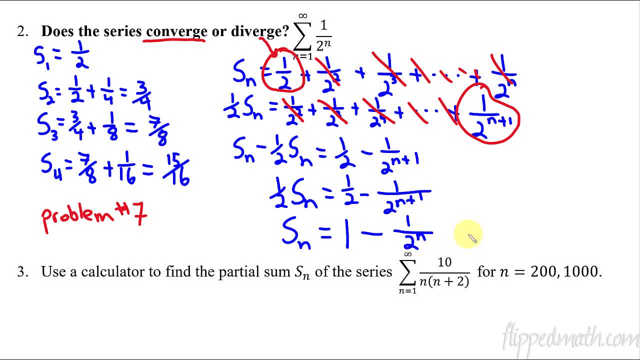 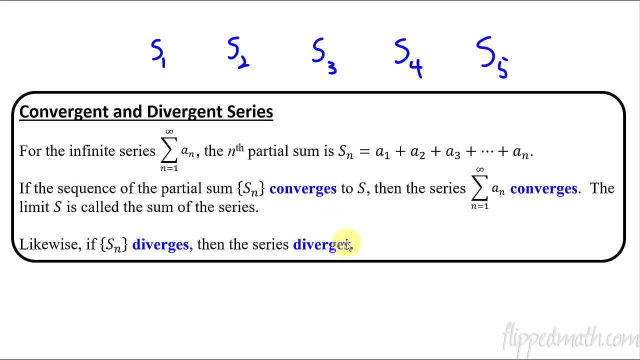 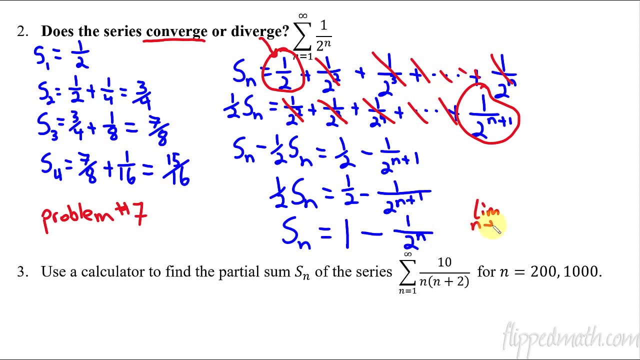 now that's important because this is now s of n. and what can i do if i want to figure out what the series is from one to infinity? you just take the limit as n approaches infinity. so if you have this approach infinity, the limit as n approaches infinity of s of n is going to equal this portion. 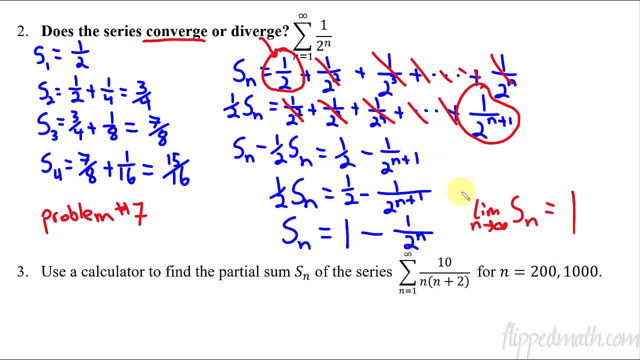 this fraction becomes a zero, so it's just one minus zero and it equals one, so it converges to one, just like we thought it did from here one half three, four, seven, eights, fifteen, sixteenths, getting really close to one, but this is the proof of exactly how you do it. so, uh, there will be a. 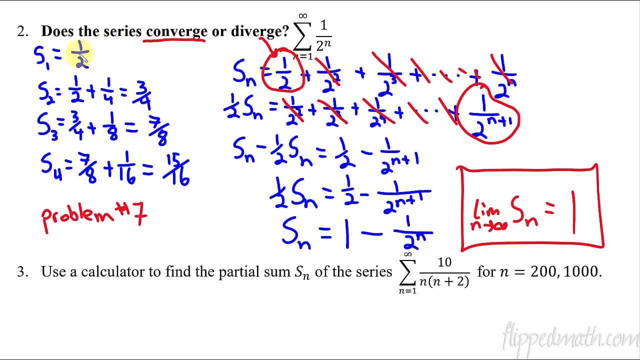 problem again that you have to do it this way. but a lot of times for these problems you could just start writing out the partial sums and be able to figure it out that way. the next part: we're just going to practice with a calculator how to plug this stuff in. so if i want to know what is s of? 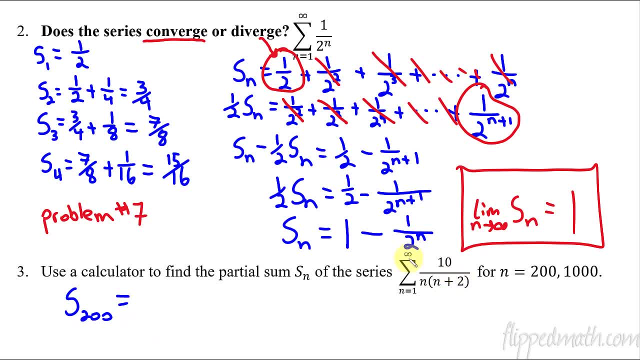 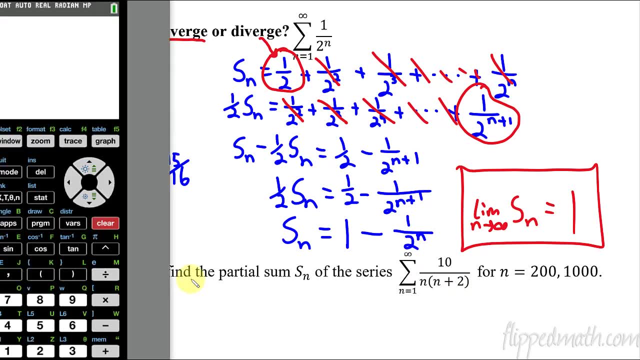 200. what does that equal? that would be adding up the first 200 terms of this sequence. well, that's going to take forever, so let's use a calculator to do that. uh, grab your calculator. and now, if you don't have a ti-84 you. 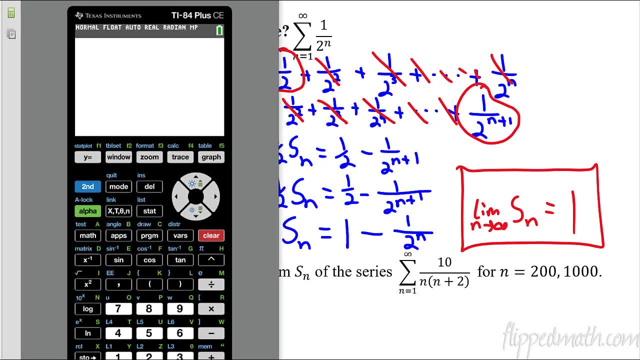 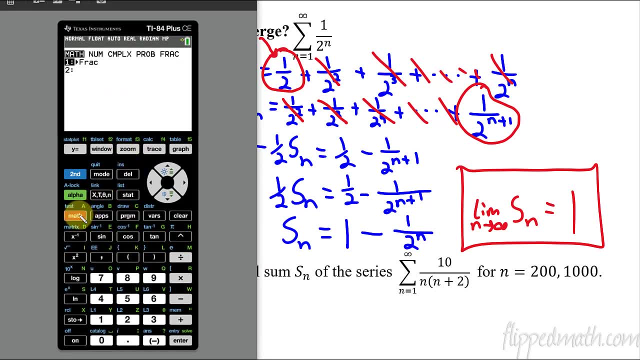 will have to look up how to do this. my apologies, i can't do it on every possible calculator out there. let's make this small enough so you can see in the screen, all right. so how you do this is on my calculator. it is math. you know how we do math eight, math nine for derivatives and integrals. 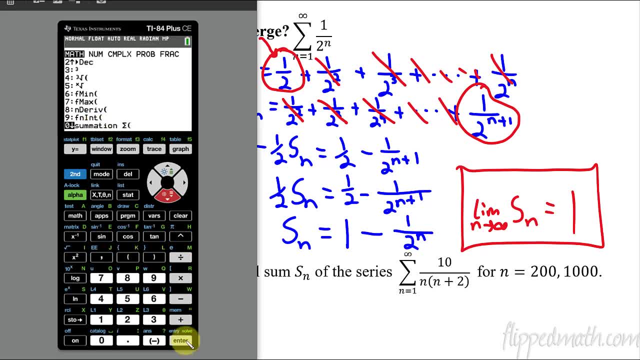 well, down here at math zero, math zero is summation. awesome, there it is okay. so again, if you don't have an 80, a texas instrument, that's okay. just look up how to do a summation and you'll see that summation notation on your particular calculator. so just google that so you make sure you can do this. 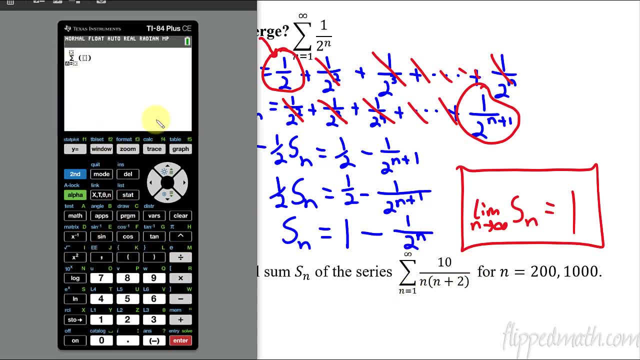 and then we're going to say the n equals. so here we have n equals. so we're going to say a variable, so the variable button is there, and we're going to go from 1 up until 200, and then we have to type out the a sub n, so it's 10 divided by. now be careful here. you want to make sure you get that. 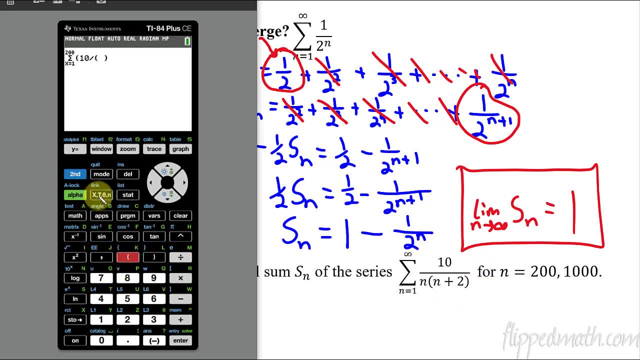 whole uh denominator in there. so i'm going to distribute the n and make it x squared. instead of an n it's x, x squared plus to x. so i just distributed it to make sure that i don't make any mistakes with my denominator. and there we go: 7.4503, so the first 200 terms add it all up together is 7.45. that's weird, huh, you'd. 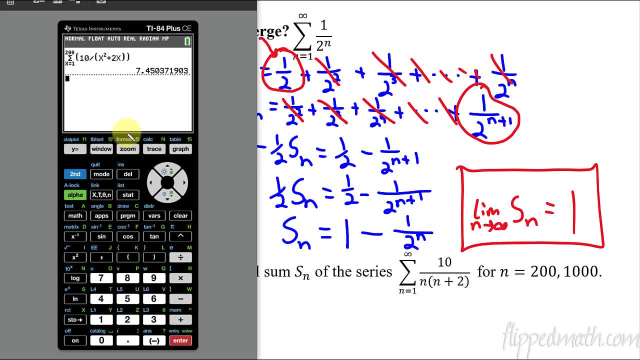 think it'd be bigger, but it's not, because you have a fraction here and so the numbers you're adding are getting smaller and smaller. now. now we'll do it up to a thousand. so i'm just going to go second enter, because that'll give my previous entry, and then i can just scroll over here, click, click, click. 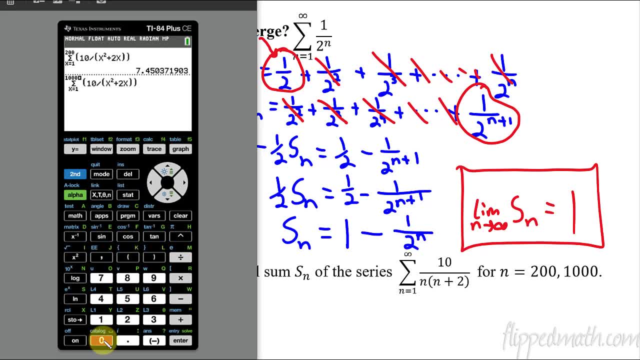 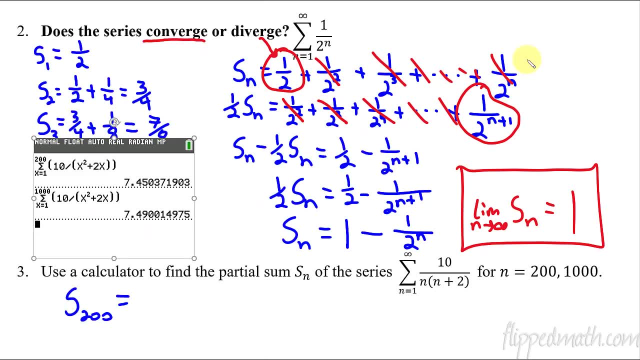 click, change this 200 to a thousand. that's a hundred thousand. hit enter. and what is it? 7.49. let me copy that over here. all right, so the 200 was 7.45. i'm going to just do a couple more decimals: zero, three and then the first thousand terms, the sum of the first thousand terms, that partial sum. 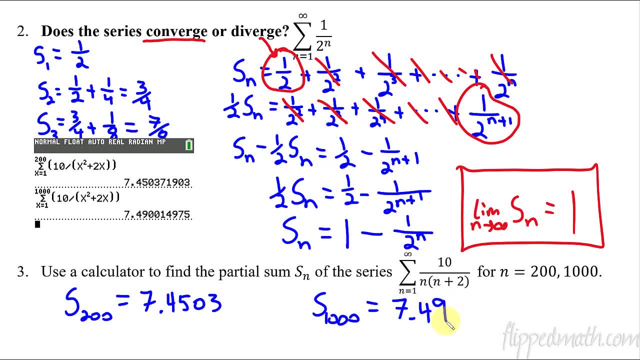 would be 7.49. so you can see, it looks to be that this, this uh series, is probably a little bit bigger than the first one, and if you guys are interested in the question about the number of many of these, you can see that the number of numbers is going to go up to 7.5. 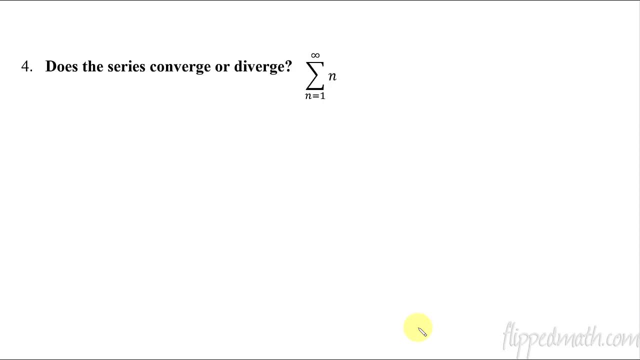 we could do even larger numbers, and you can see it's going to get closer and closer to 7.5. so that's a way you can use a calculator to help you figure these partial sums out. uh, pretty quickly. and our last problem: this one's going to be pretty quick and easy, that is, does this one's? 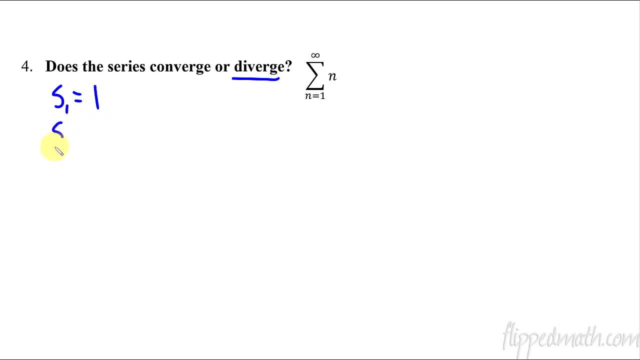 converge or diverge. well, i'm giving you one that diverges, just because i wanted to make sure you saw what happens. so the first term- let's look at this first term of the first two- is going to be one plus, and now we plug in a two. well, that equals three. the next: 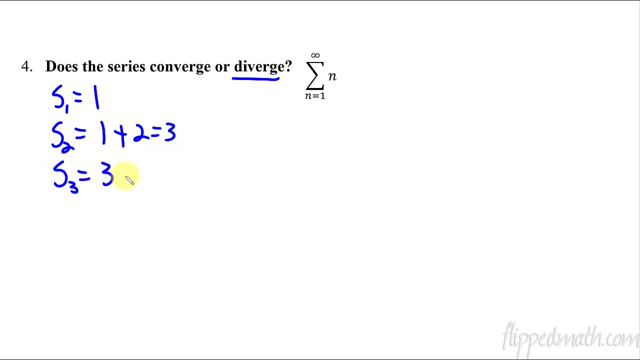 one. the first three is going to be the first two added together, which is three plus plug in a three. so then that equals six. all right, let's do the next one: four, so that's going to be the first three terms, which is six plus plug in a four. okay, that equals ten. what's the fifth one? fifth one is: